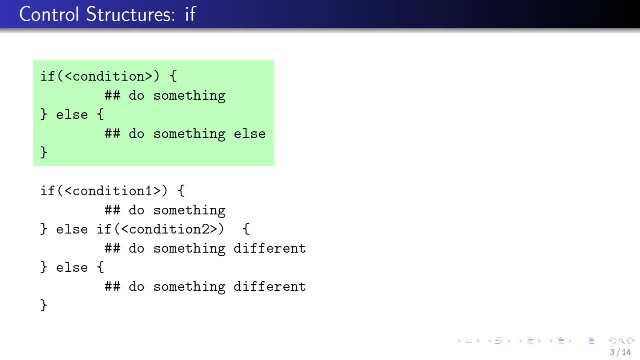 kind of construct. The else part is optional, so you could just have an if statement to do something, if something is true, but you can have the else part if you want to do something. alternatively, If you want to do more, if there's more, 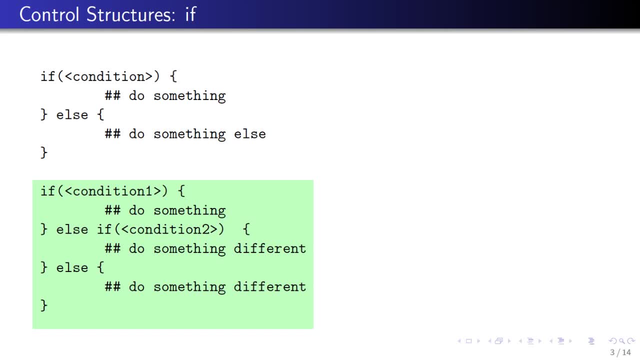 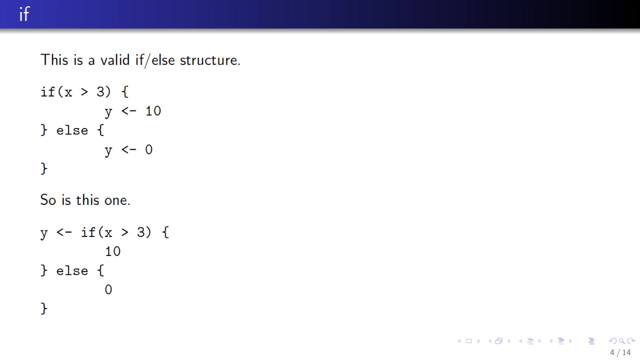 than one possible type of condition you want to check. you can say if and then else, if and then else Else, if there can be any number of else, if conditions in a construct like this and the else one has to be at the end. So there are a couple of different ways that. 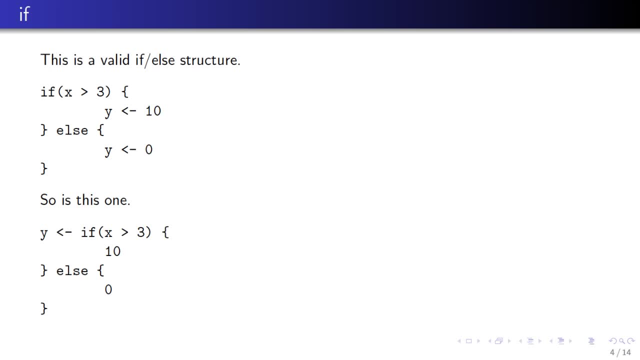 you can formulate the if else construct in R. This is a little bit different from other languages, in case you haven't seen something like this. So the first is pretty standard. If the symbol x is a is greater than 3, then you set y equal to 10.. 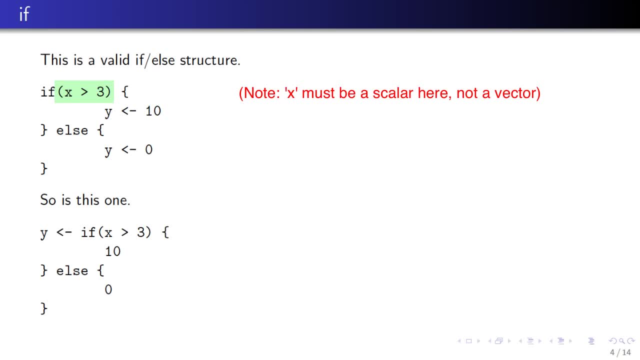 If it's not greater than 3, then you set y equal to 0.. So that's inside the if-else construct. there's an assignment of y to a specific type of value, depending on what the value of x is. But, however, in R you can do it a different way. 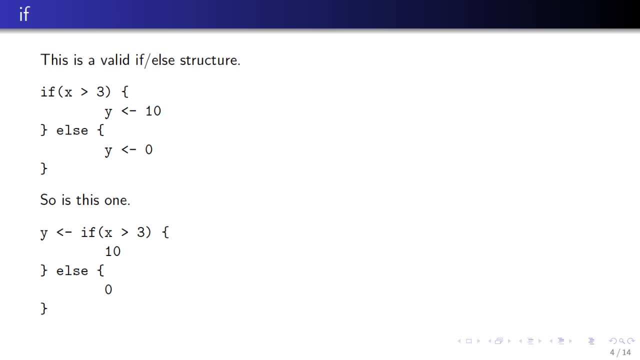 You can say: y is equal to the entire if-else construct. so if x is greater than 3,, 10, or 0, depending on whether that condition is true or not, So this is a valid formulation also. So sometimes it's useful to read this type of writing. 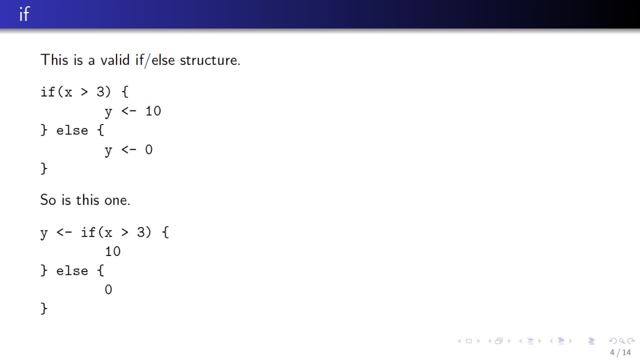 because it allows you to realize that the entire if-else construct is all about assigning a value to y. So, as I said before, the else clause is not really necessary. You can always test a condition and do something and then do nothing if that condition happens to be false. 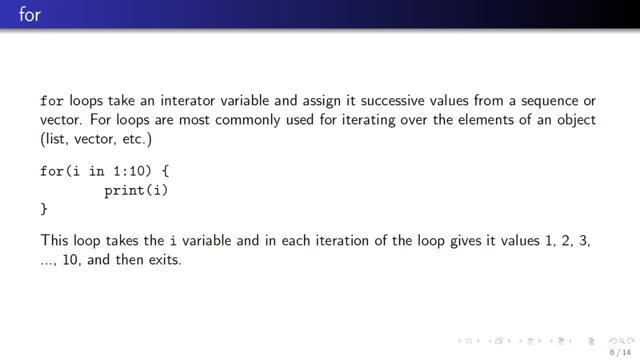 And you can just test multiple conditions in a row if you want. So the next construct is a for loop, So this is probably the most common type of loop operation that you're going to use in R. The basic idea is that you have a loop index. 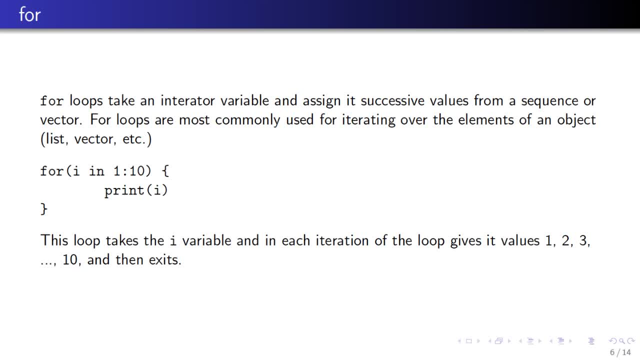 which is typically called i. but if you have many loops you might say j, k, l, etc. And a loop index is going to cover a sequence of numbers, typically integers. So for example, here I've got a for loop. 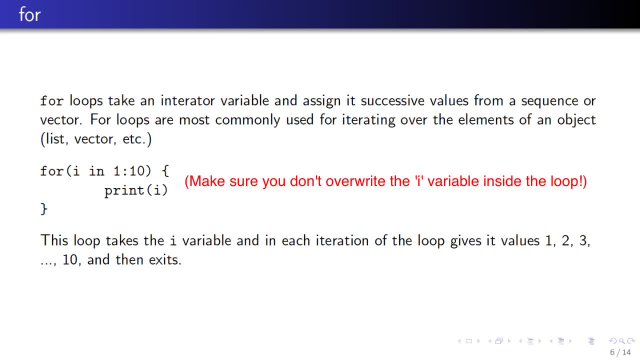 and it's looping over the numbers 1 through 10.. So I've created the sequence of the colon operator 1 through 10.. And this for loop is not doing anything particularly interesting, It's just printing out the numbers. so I'm printing out i. 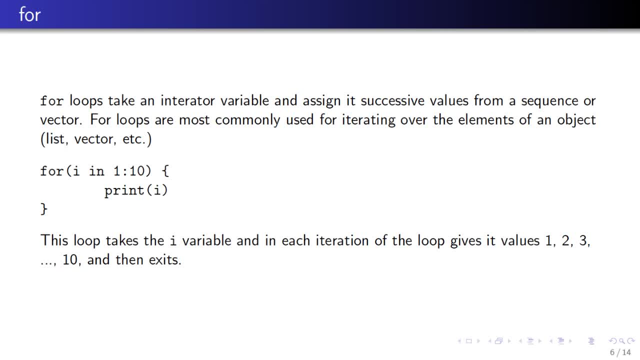 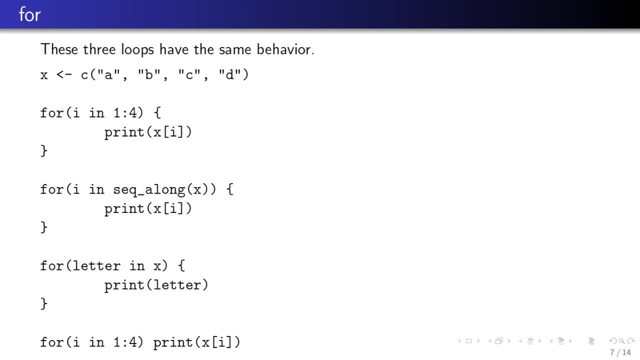 at each iteration. After the loop is finished it continues on to the next block of code. So there's different ways to use a for loop And R is pretty flexible about how you can kind of index the different types of R objects. So here I've created a vector, a character vector. 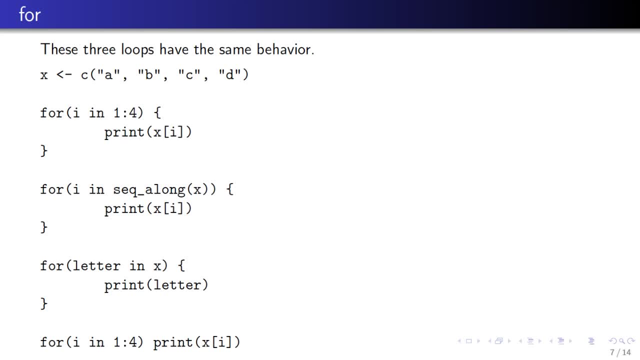 with the letters a, b, c, d in it, And all of these for loops are equivalent. So for example, the first one, I kind of done what you might commonly see in other languages like C that have for looping. Here I've got an index. i. 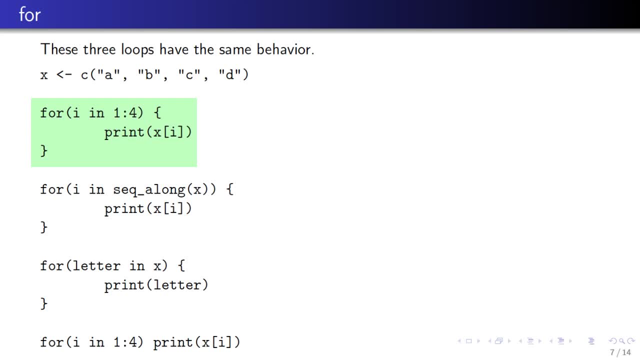 that I sequence through 1 through 4.. I create an integer sequence And then I print out the ith element of x each time. So here this loop just prints out a, b, c, d. Another thing I can do is use the seek along function. 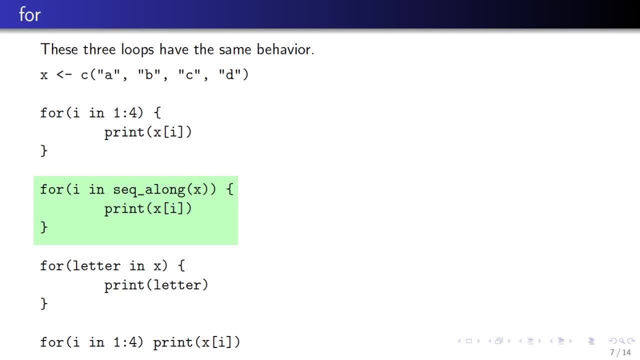 So seek underscore along. What it does is it takes a vector as an input and it creates an integer sequence that's equal to the length of that vector. So this is a vector of length 4.. So it's going to create an integer sequence. 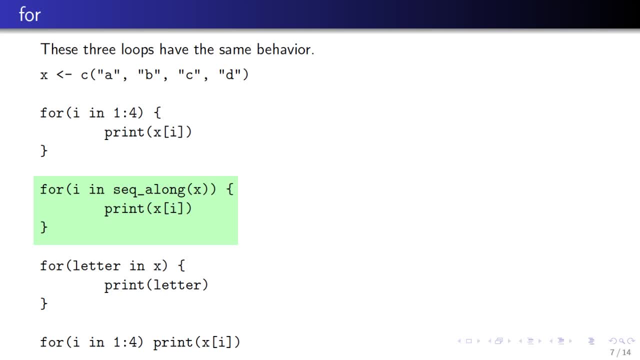 of 1 through 4.. It's exactly the same as the previous statement where I've got the sequence 1, colon 4.. However, here I generate the sequence based on the length of the variable x. So now my index variable. i is going through this sequence. 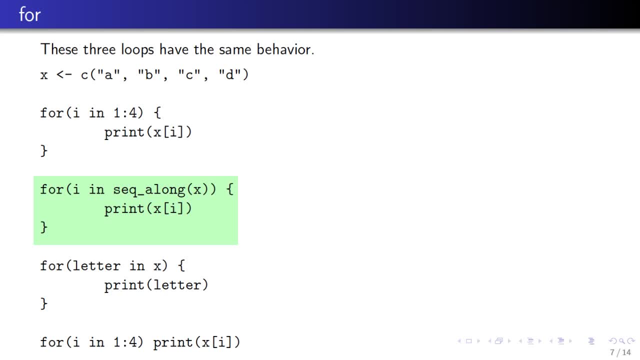 It's printing out the ith element of x And exactly the same behavior occurs. I print out a, b, c and d. The third example: here I've got a different index variable, I'm calling it letter And the index variable is actually going to be. 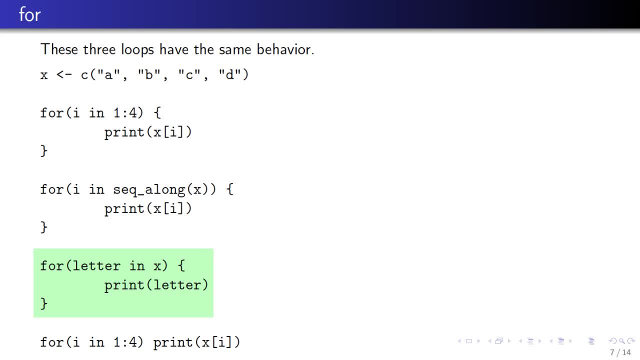 indexed to the length of the variable. So I'm going to print out the index variable And the index is going to be taking values from the vector itself. So there's no reason why the index variable has to be an integer. It can take elements from any arbitrary vector. 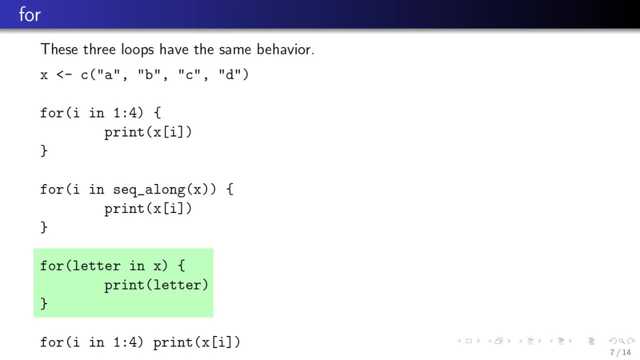 So now the for loop is going through this vector of letters a, b, c, d, And it's just going to print out the letter itself. So now I'm printing out the index variable, which happens to be equal to the letters in the vector. 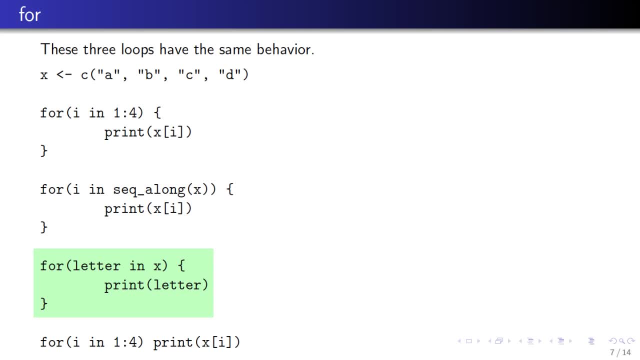 And so these three for loops are exactly the same so far. The last version here is the same as the first one, except that I haven't included the curly braces, And so for a single expression if the for loop only has a single expression in its body. 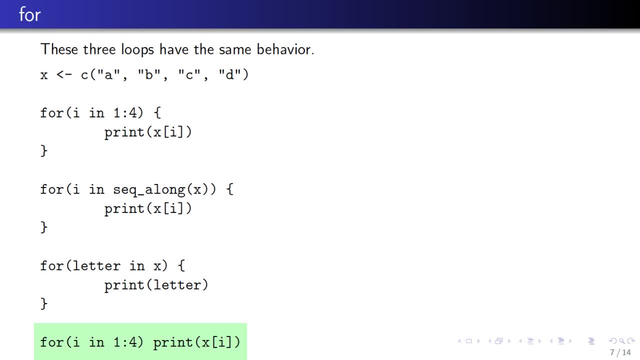 you can omit the curly braces and put everything on one line, which may be useful sometimes because it's a little bit more compact, But it's not my particular style For for loops. I generally like to put the curly braces in, regardless of how many elements are in the body. 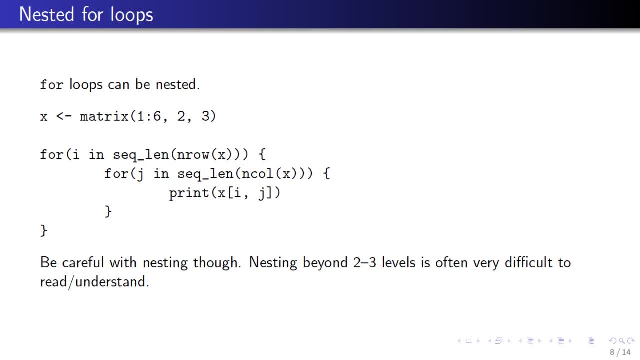 For loops can be nested, So you can have a for loop inside of a for loop. So the common thing, for example, is with a matrix that has two dimensions, and then you might want to loop over the rows and then loop over the columns. 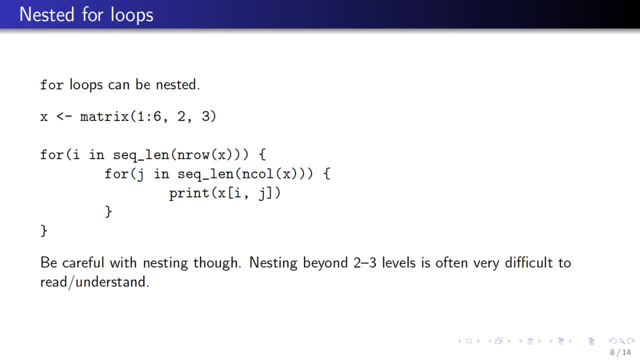 So here the outer loop with the i index is looping over the rows And I'm using a function that's called seek underscore len. So the idea is that it takes the seek underscore len, takes an integer, which in this case happens to be the number of rows in x. 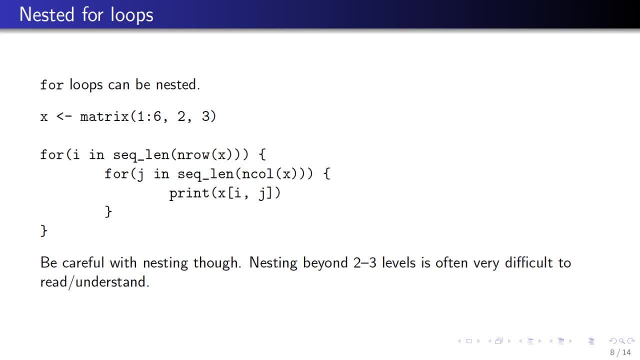 and it creates an integer sequence out of that. So, if so, this particular matrix has two rows, And so it's it's going to create the sequence 1 to 2.. Similarly, the nested loop with the j index is using the number of columns to create a sequence. 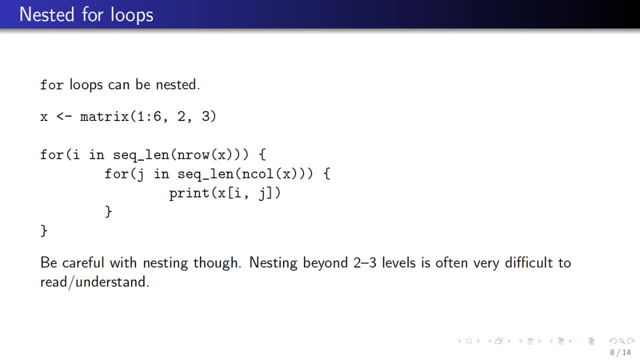 So this matrix has three columns, and so the seek underscore len function is going to create an integer sequence, 1 through 3.. So this doubly nested for loop is basically printing out all the elements of the matrix. So one thing to be careful with nested for loops. 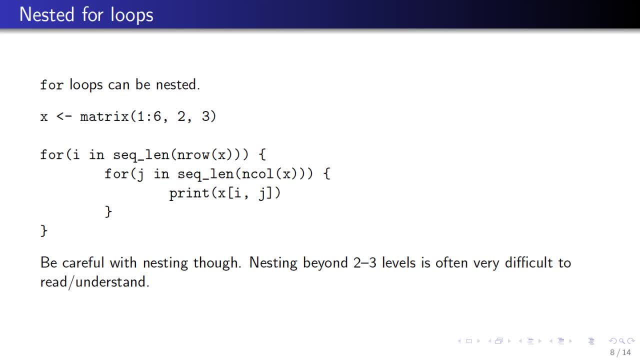 is that it's going beyond 2 to 3 levels. while it's theoretically okay in R, It makes reading the code a little bit difficult to do, And so if you're reading code that has three or four nested for loops, it gets difficult to understand what's going on. 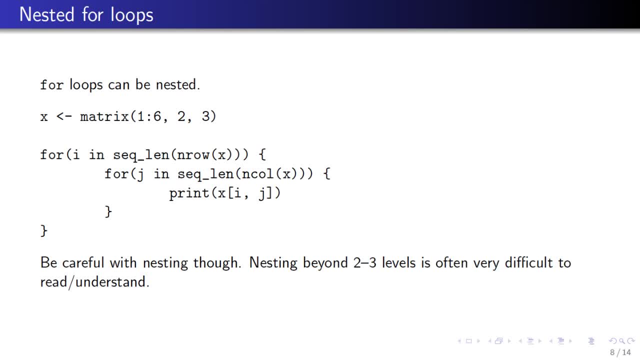 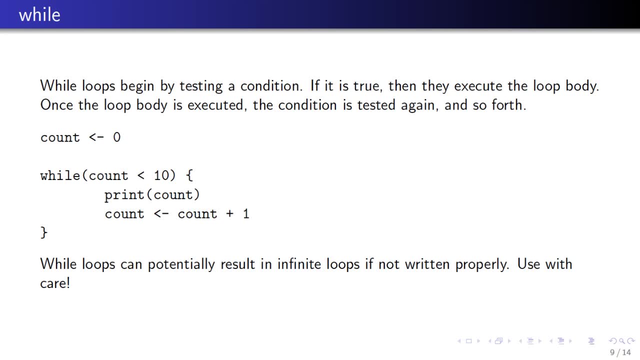 Sometimes that's a logical thing to do, but many a times there's ways to get around that, for example by using functions. So the while loop is the other major looping construct in R and the basic idea is that the while takes a logical expression. 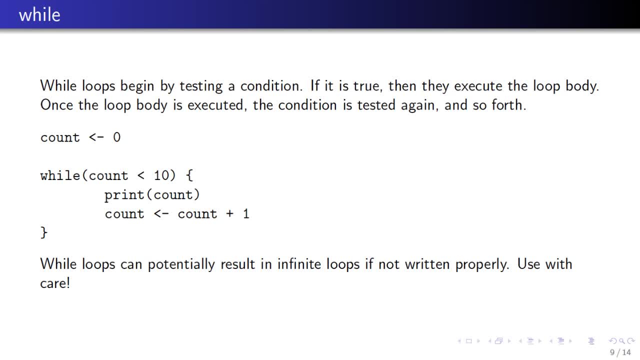 that's going to create a sequence 1 to 3.. And we'll execute the loop based on the value of that logical expression. So, for example, I've got a very simple loop here. It initializes a count variable equal to 0,. 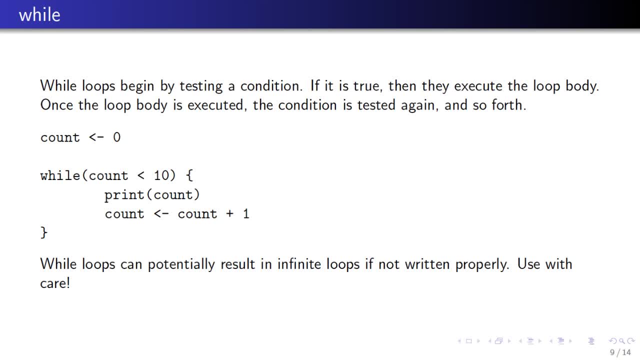 and then, while that count is less than 10, it prints out the count and then increments the count by 1. So as soon as the value of count gets to 10, the loop stops and then it'll go on to the next body of code. 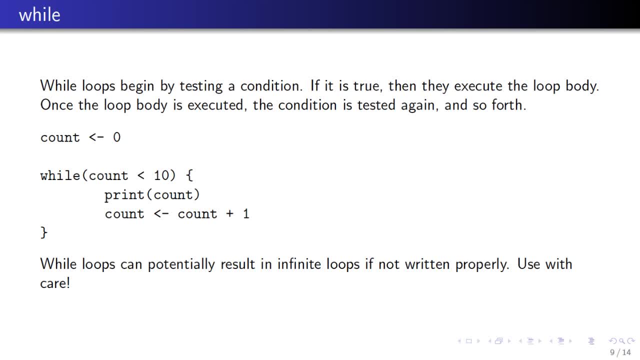 So the while loop is useful because it makes things easy to read sometimes. It's very obvious here that this loop is supposed to stop working or stop executing when the value of the count variable is 10 or more. So it makes it a little bit more readable. 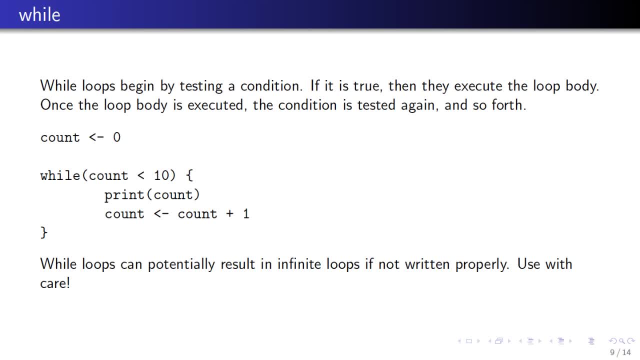 However, you have to be a little bit careful with while loops, because, technically speaking, they are infinite loops and you have to make sure that the condition that stops the loop will actually occur. Otherwise, your program will never finish, And so, in this case, 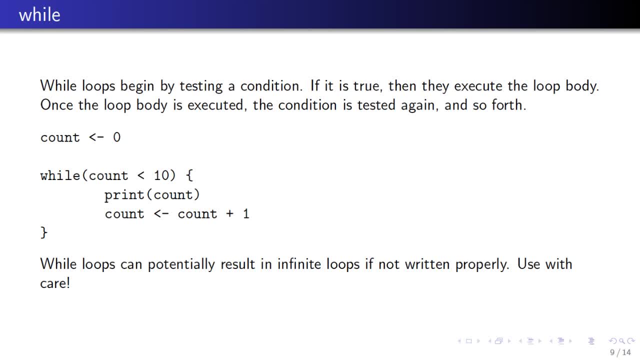 it's fairly obvious that the loop will eventually stop executing, But in much more complex pieces of code it can be hard sometimes to figure out whether the while loop will finish, And so often it's safer to use something like a for loop that has a hard limit. 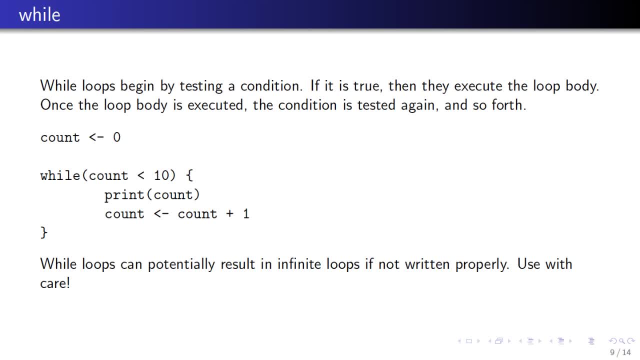 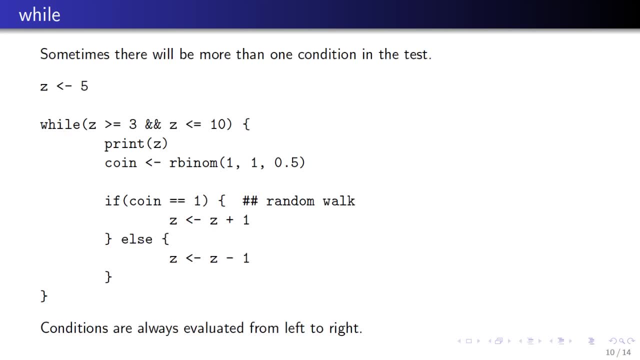 on the number of times it can execute. So it's not necessarily saying that you should never use a while loop, but you just have to be careful when you do use them. So you can test multiple conditions in a while loop or in any type of construct. 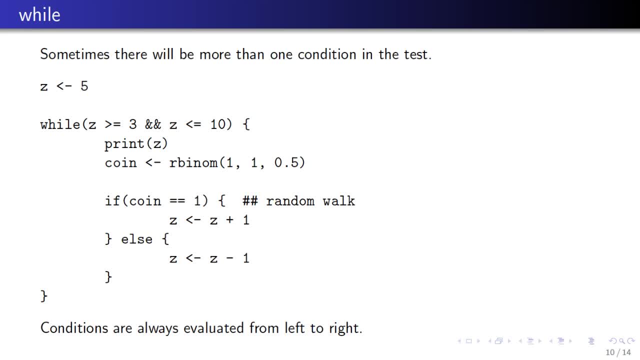 like an if statement, for example by using the logical operators. So here I've got. I've got a variable z which is equal to which I initialized to the value five, And the condition for the while loop is basically: while z is greater than or equal to three. 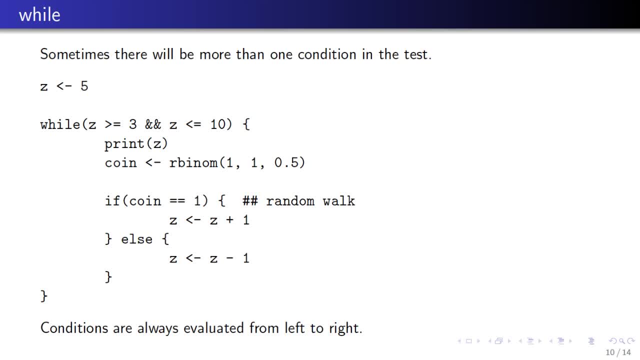 and it's less than or equal to 10.. So, while it's between the values of three and 10, then what I'm going to do is going to print the value of z. I'm going to flip a coin, a fair coin. 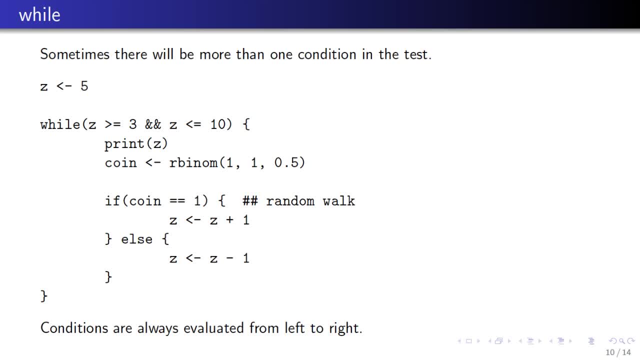 And if the coin is a one, I'm going to add one to my value, And then if it's less than one, sorry, excuse me- if the coin is equal to zero or any other value for that matter, I'm going to subtract one from z. 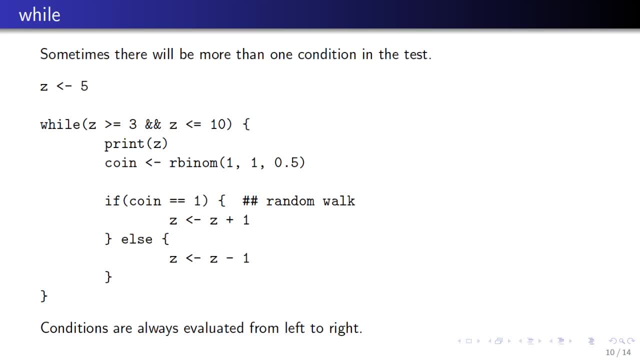 So this is. I'm generating a little random walk here and the value of z is going to go up or down depending on my little coin flip here, So when? so here you can see it's a little bit harder to tell when the while loop will finish. 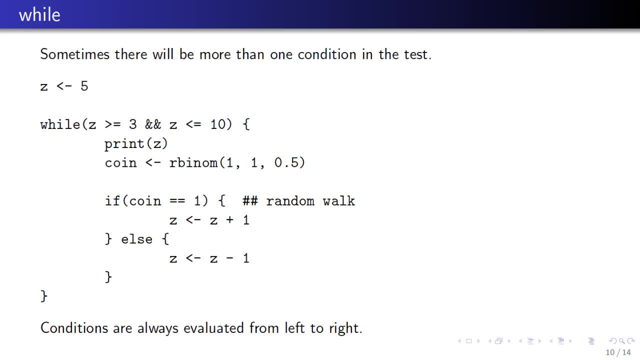 because the body of the while loop involves random number generation. So here the z value is going to zigzag up and down until it eventually hits 10, or eventually it hits three or something less than three, And so this may be kind of nice. 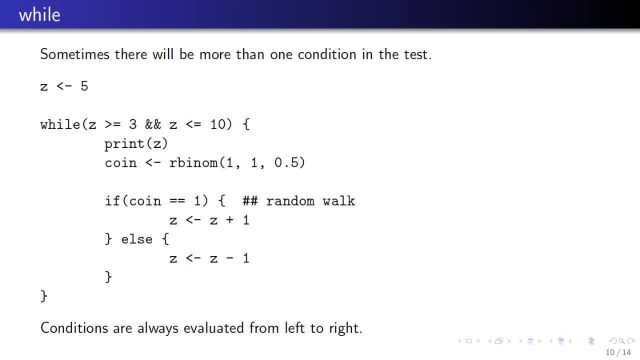 but you have to be careful that it doesn't go off for too long. So one thing to note on a more technical level is that the conditions in a in any when R tests the condition in a multi, in a kind of a multi-expression condition. 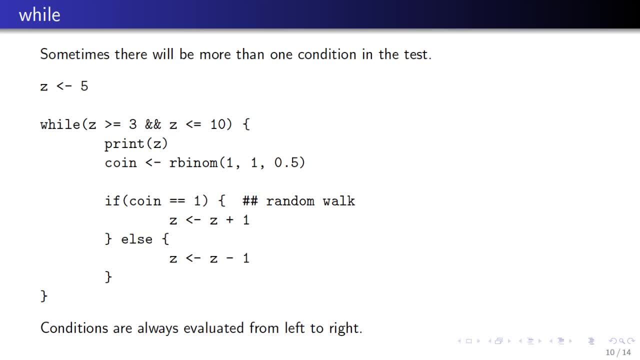 here I've got z greater than or equal to three and z less than or equal to 10, the conditions are always evaluated from left to right, So it checks to see if the less, if the less most condition is true, and then it goes to the next condition. 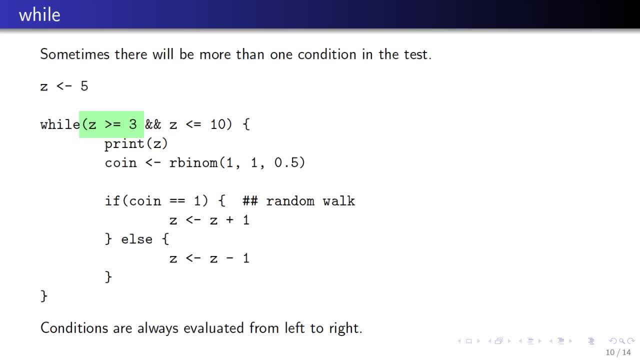 So first it'll check to see if z is greater than or equal to three. if that's true, Then if that happens to be true, it'll go to the next expression and it'll say: it'll check to see if z is less than or equal to 10.. 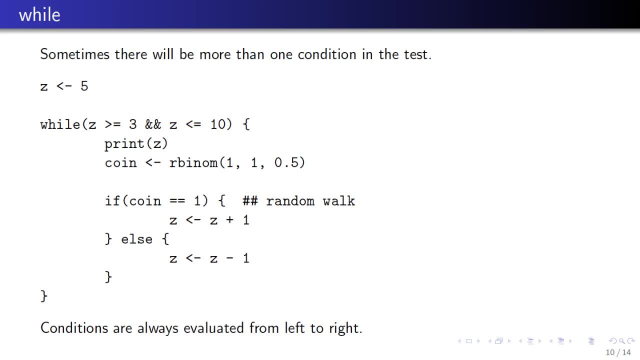 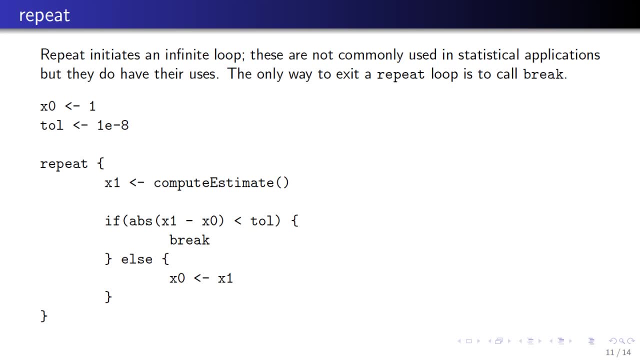 So then there, if those are both true, it goes on to the next, into the body of the loop. Repeat is a construct that basically initialize, initiates an infinite loop. This is not a what I would characterize as a commonly used. 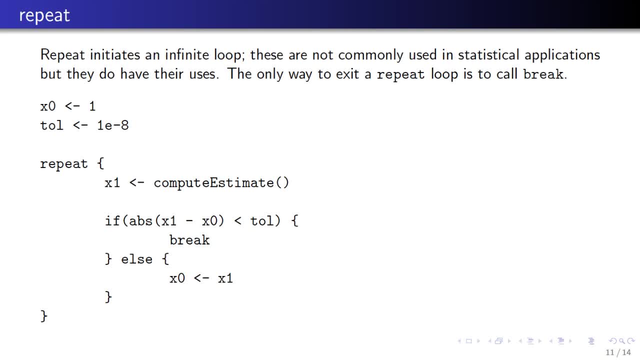 control structure in R, but it does have its use occasionally. So the only way to exit a repeat loop is to call break. So obviously you're going to have to call break at some point, unless you feel like running your program, you know, forever. 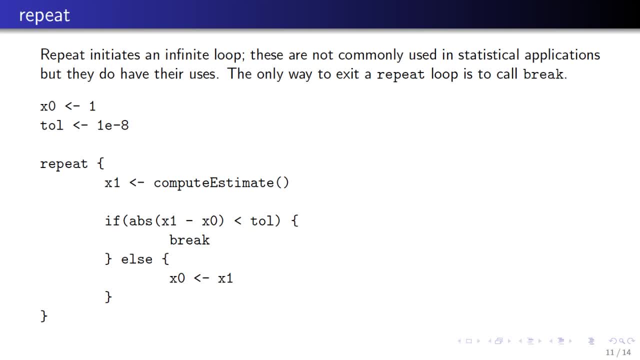 So here is a pretty simple example. Here I'm initializing at a value of x, zero to be one, and I'm setting what's called what I think of as a tolerance to be 10 to the minus eight, And then I'm going to repeat the following structure: 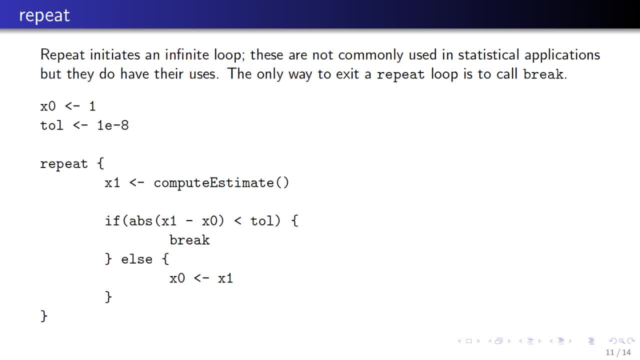 Basically, I'm going to imagine that there's some function that computes an estimate for x and I'm going to call that x one. And basically, if the new value of x, that is, x one, is if the absolute value of the difference between x one, 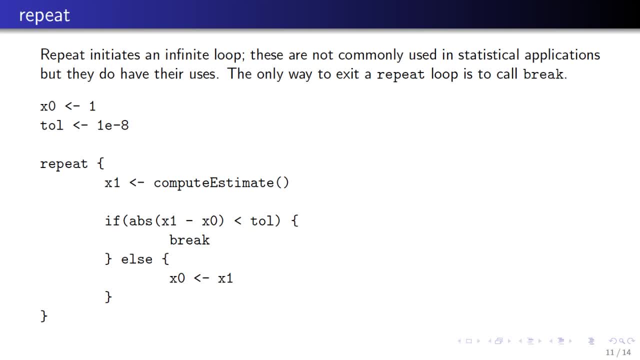 and x zero is less than some tolerance, in this case 10 to the minus eight, then I'm going to stop the loop and then move on to the next bit of code. If the difference is greater than my tolerance, then I set x zero to be equal to the new value. 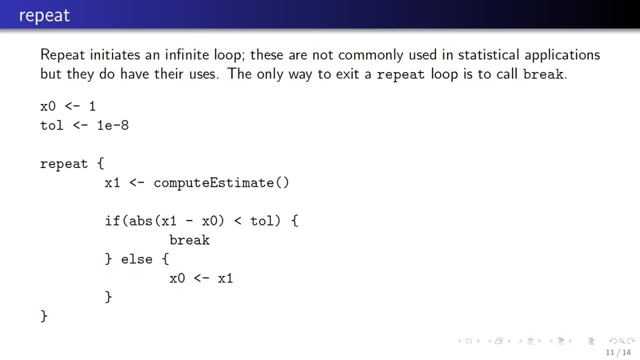 and then I run the loop again, I calculate a new estimate and I check to see if the difference is small. So this is a common type of formulation in many types of optimization algorithms, For example, if you're trying to find the solution, 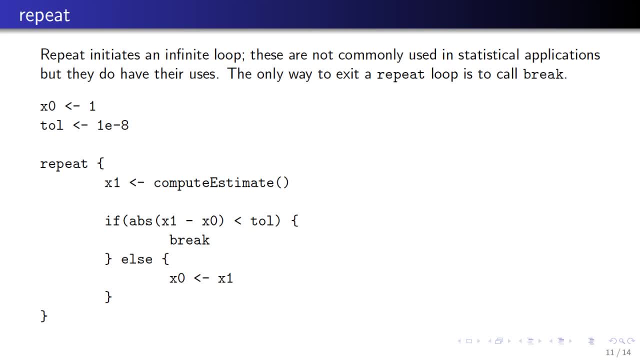 to some set of equations or you're trying to maximize a function. often you'll iterate over and over again and you'll stop when the estimate or the minutes that you're calculating are getting closer and closer together, because that's usually a sign. 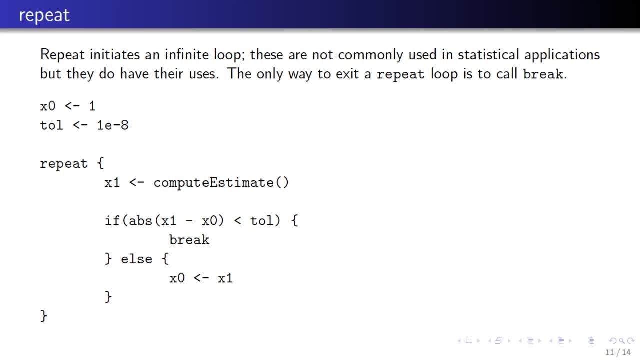 that you're kind of converging to whatever the minimum or maximum of the objective function is. So in theory, this is a perfectly reasonable construction. You want to keep recycling through the algorithm until the two values are close. So there's one problem, which is that 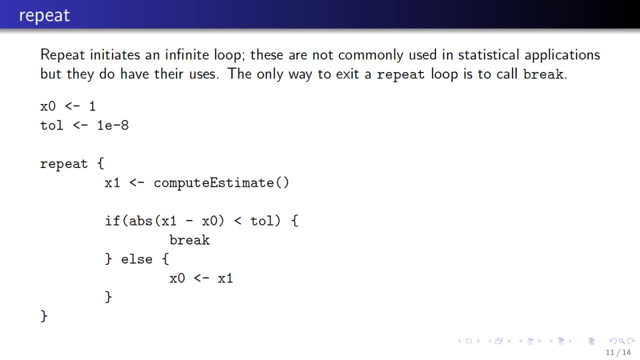 first of all, it requires an algorithm that is guaranteed to converge, and not necessarily every algorithm has that property. Second of all, it does depend a little bit on the tolerance whether the loop will run longer if the tolerance is smaller. generally speaking, 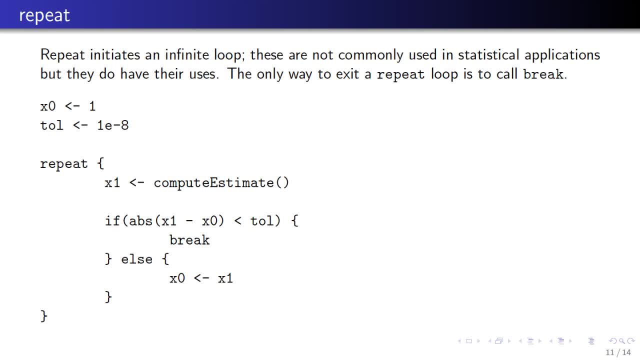 And because it's hard to predict how long this loop will run, it can be a little bit dangerous because it's unpredictable. it could theoretically run forever and you have no way to guarantee that the program will stop at some point. So this construct, although it's theoretically, 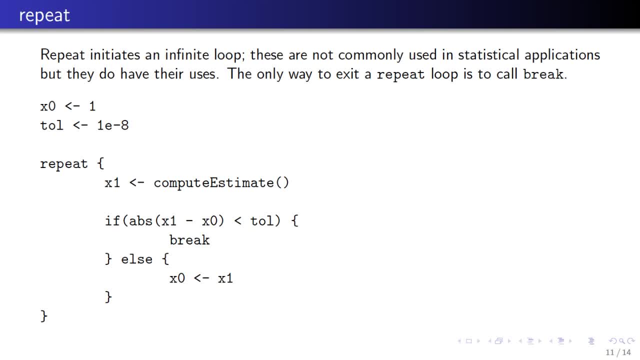 kind of the right thing to do. it's usually not a good idea. It's probably better off to use a for loop that has a hard limit on the number of iterations that it's allowed to run. That way, if you have a problem with your algorithm. 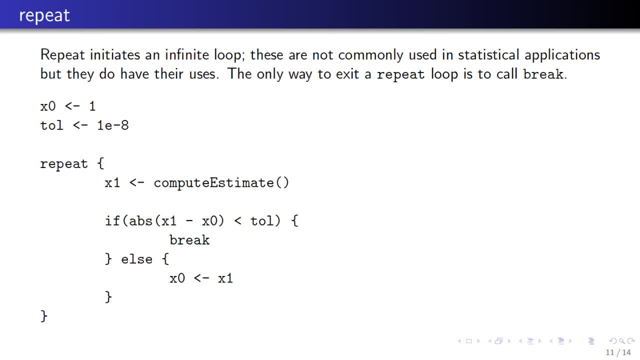 it will eventually reach the hard limit and stop, and you'll know that the reason it stopped is because it didn't converge. and then maybe you can try to fix something about the algorithm With the repeat type of approach if your algorithm is not converging. 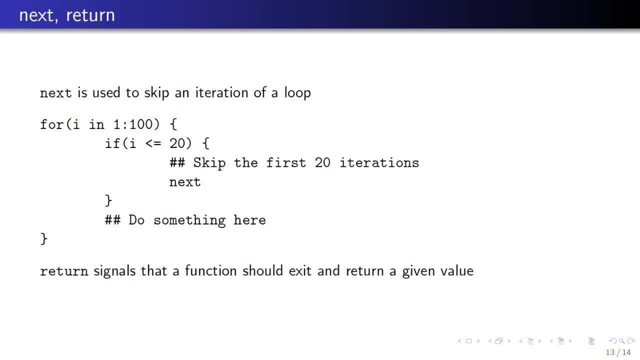 you won't have any warning, it'll just be running a really long time. The last control structure element I want to talk about is next, and then there's also return. Next is basically used in any type of looping construct When you want to see if there's a loop. 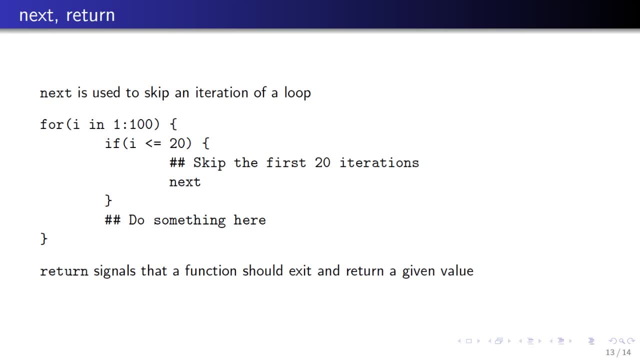 you want to skip an iteration. So here I've got a basic for loop which is going to run for 100 iterations, but the idea is that I want to skip the first 20 iterations and then only kind of execute some code for iterations 21 through 100. 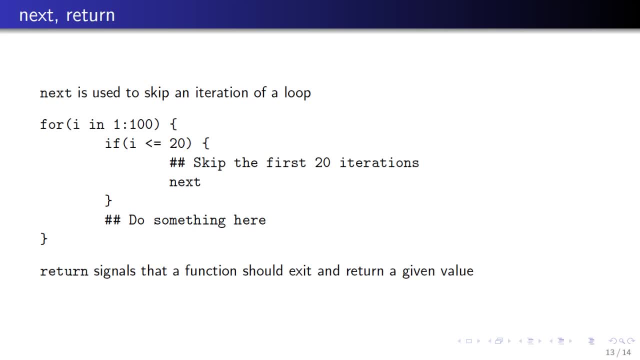 So here I've got a very simple if condition. so if i is less than or equal to 20, I'm just going to skip. So I use the next expression and it'll skip everything else in the for loop and iterate again. 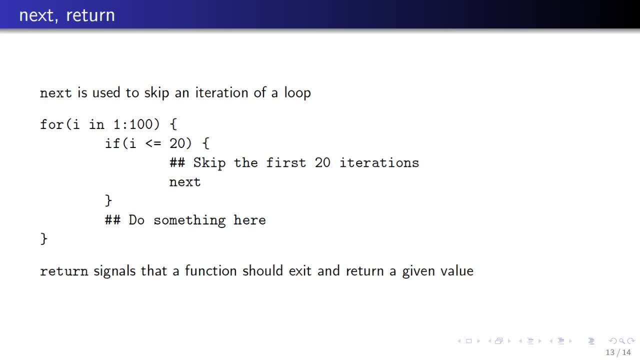 So once i gets beyond 20, then of course the expression i less than or equal to 20 will be false, and so it won't execute the next it'll go into whatever the body of the code for the for loop is. So next is a way to skip an iteration in a loop.